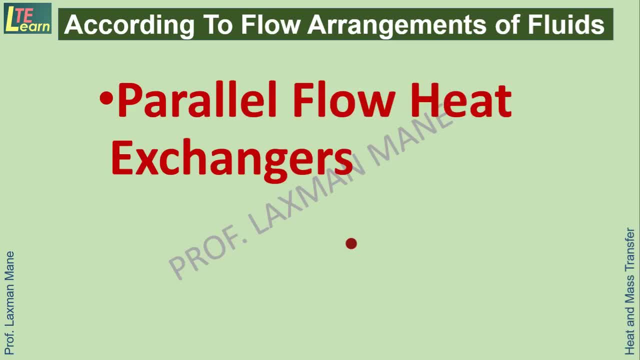 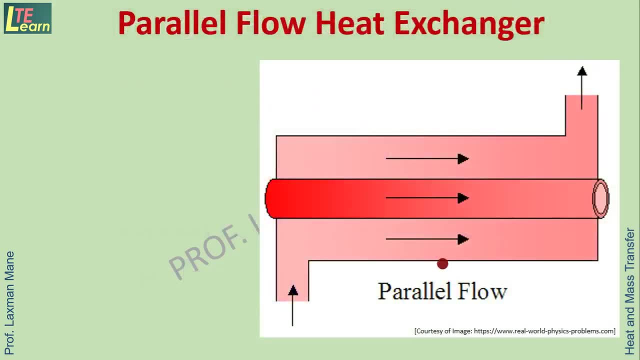 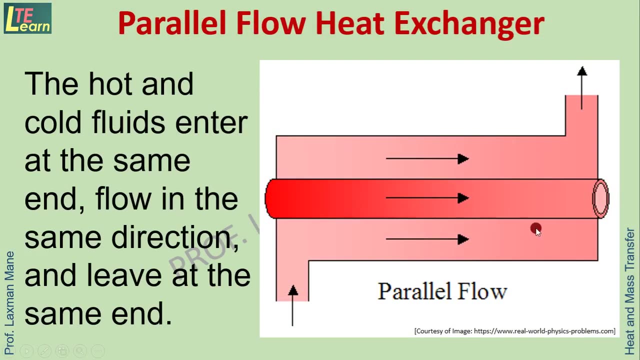 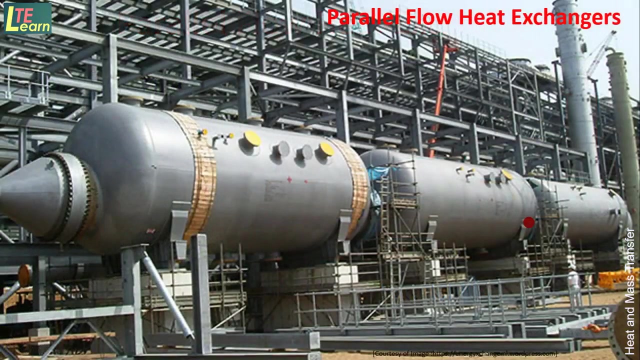 are classified into two types: parallel flow heat exchangers and counter flow heat exchangers. in parallel flow type heat exchanger the hot and cold fluids enter at the same end and flow in the same direction. means here we see, these are moving in parallel with each other and these fluids live at the same end. 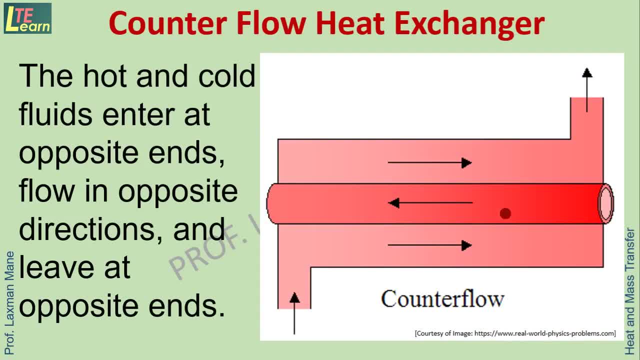 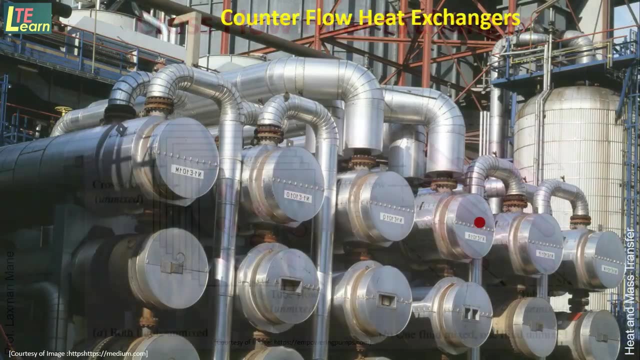 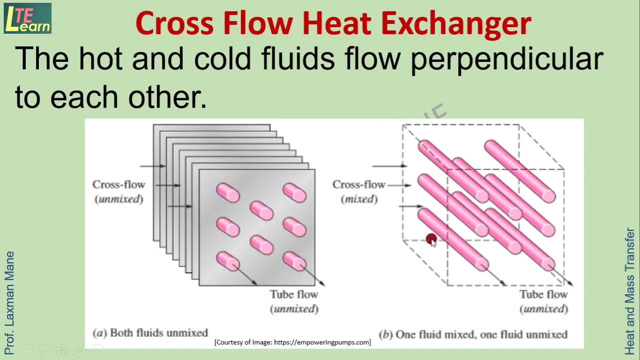 In counter flow heat exchanger the hot and cold fluids enter at opposite ends and flows in opposite directions and live at opposite ends. In cross flow heat exchangers, the hot and cold fluids flow perpendicular to each other. Here are two types of cross flow. 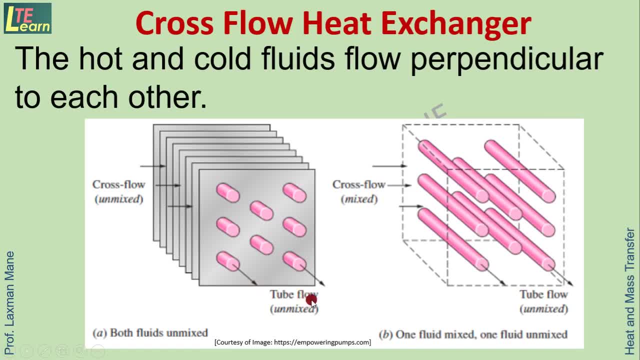 In first type, cross flow fluid and tube flow fluid. both are unmixed. They are separated By these plates and tubes. In second case, the fluid which is passing through the tube is unmixed, But the fluid which is passing over the tubes, that is mixing. 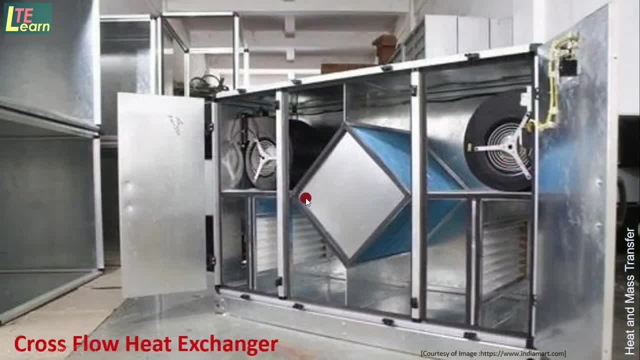 So it is mixed cross flow fluid. This kind of heat exchanger is used in air handling unit, So here air is cooled by using chilled water, So chilled water is passed through the air And air is passing over these tubes outside, So here is no direct contact between these two fluids. 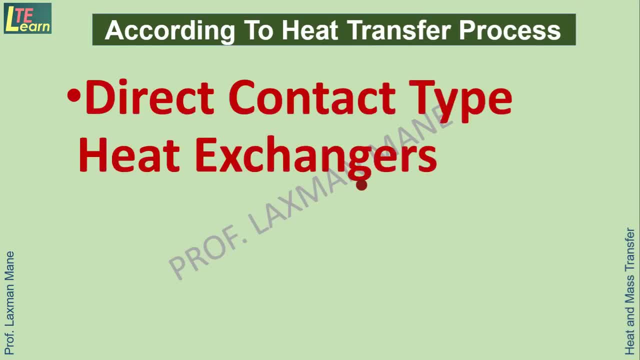 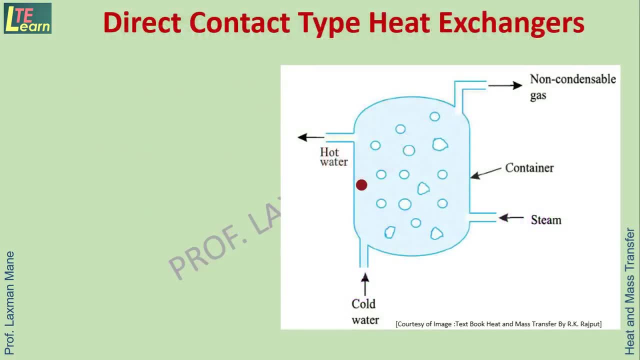 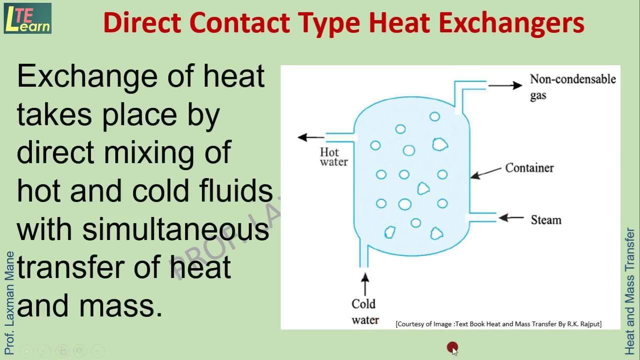 According to heat transfer process, there are two types: Direct contact type and indirect contact type heat exchangers. In case of direct contact type heat exchangers, here exchange of heat takes place by direct mixing of hot and cold fluids, With simultaneous transfer of heat and mass. 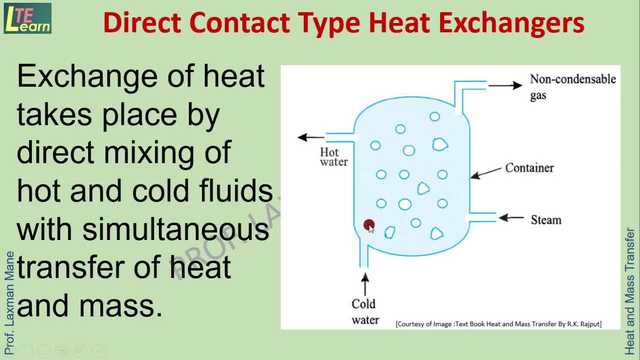 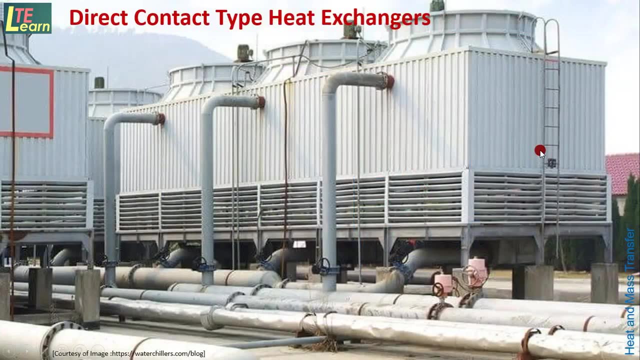 In this diagram we see this is a cold water which is passing and mixing with the steam. Both are mixing together, So cold water is becoming hot water and the steam is coming out as a non-condensable gas. So this type of heat exchanger is used in a surface type heat exchanger or condenser. 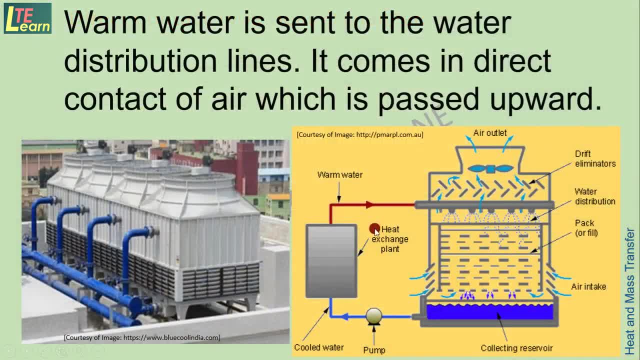 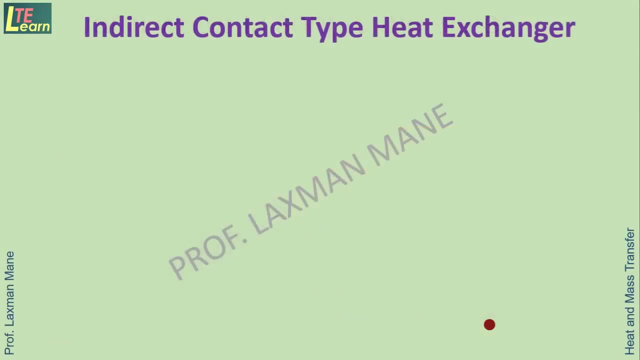 Which is used for cooling of warm water. So this is a warm water which is sent to the water distribution line, There it is sprayed. It comes in a contact with air which is moving in upward direction. So thus this warm water is cooled, that is collected here in the collecting reservoir. 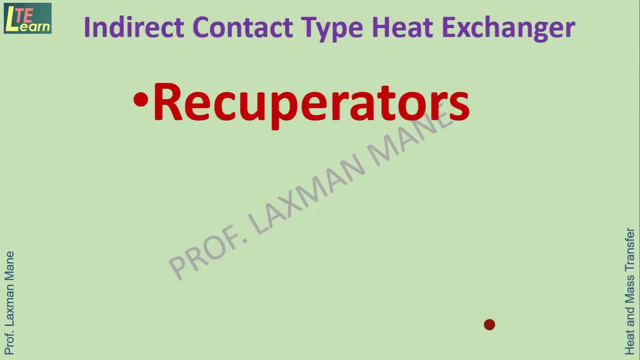 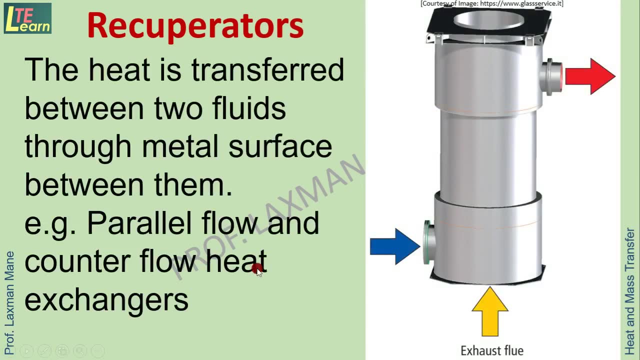 In case of indirect contact type heat exchanger, there are two types. The first is a cold water, which isorrover flow, which like in printed form- I'll explain more about it soon- And the second is a flow sort of a liquid. 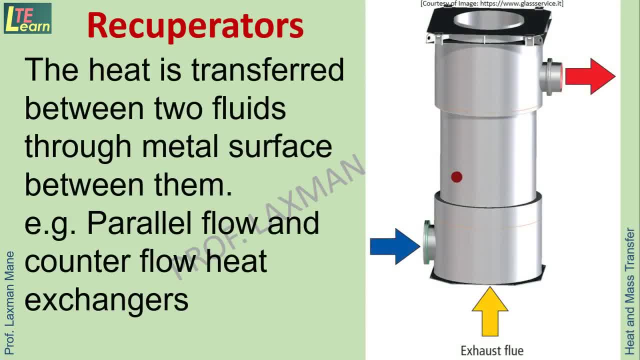 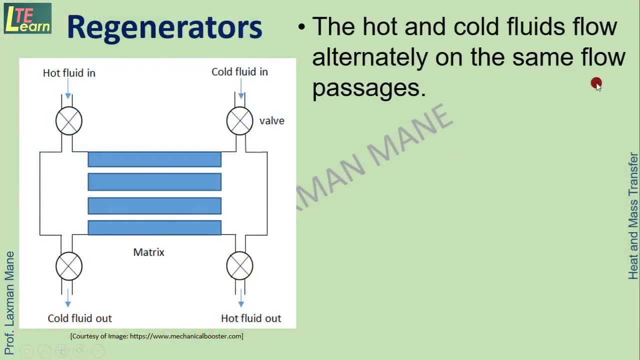 One call as an indirect feeling flow. Ti is passed to some pure pressure inside C is the current flow. Put it on heat exchanger and here till now there is a valid non-condensable flow, Because here hydrogen at low power, it will feel cool. 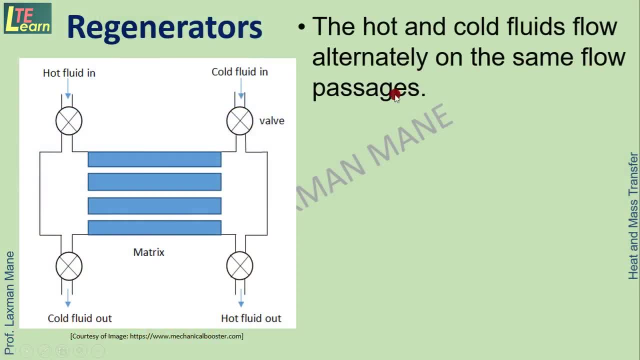 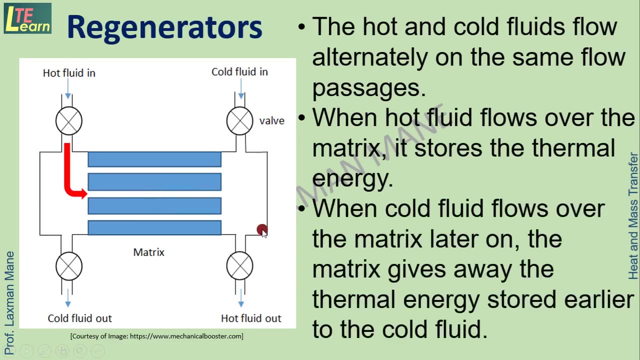 Whim minister can get excited. Tomorrow all videos will be published on the same flow passage. so first, when hot air fluid flows over the matrix- this is a matrix, it is storing the thermal energy in the matrix. then, when cold fluid is passing or flowing over the matrix later on, the matrix gives away. 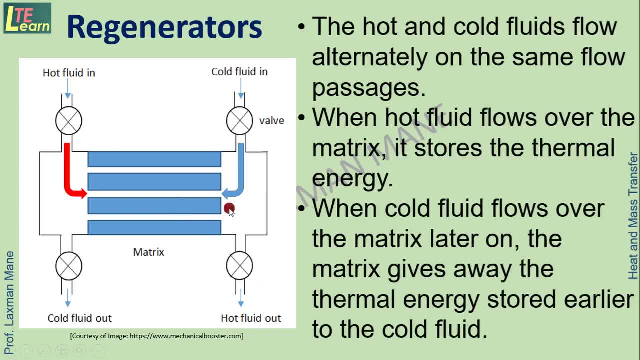 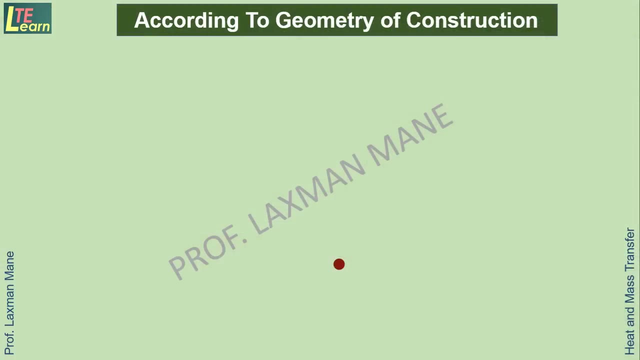 the thermal energy stored earlier to this cold fluid. so cold fluid is going inside at this point and is coming out at this point. hot fluid is going inside at this point and coming out at this point. according to geometry of constructions, these are classified as shell and tube. 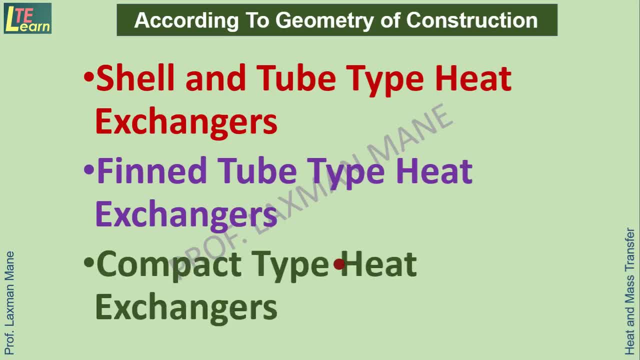 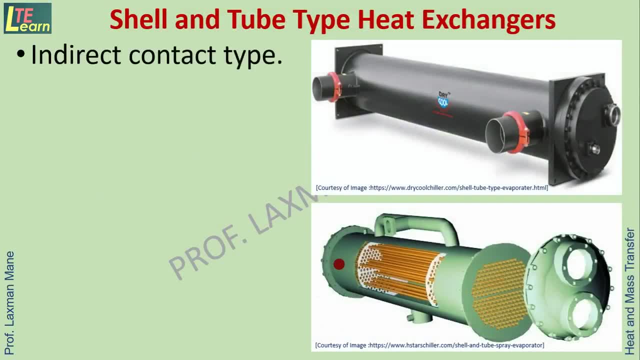 type heat exchangers: finned tube type heat exchangers and heat exchangers. shell and tube type heat exchangers and compact type heat exchangers. shell and tube type heat exchangers. it is indirect contact type in this large number of. 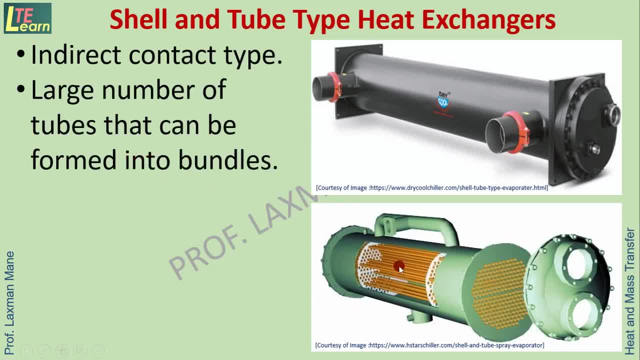 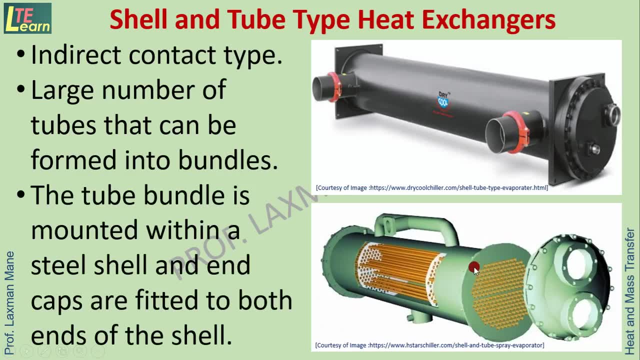 tubes that can be formed into bundles. so these are the tubes, bundle of tubes. the tube bundle is mounted within a steel shell, so this is a shell, and end caps are fitted to both ends of the shell. so this is the chili Avecell. such a Chand铆 strength. 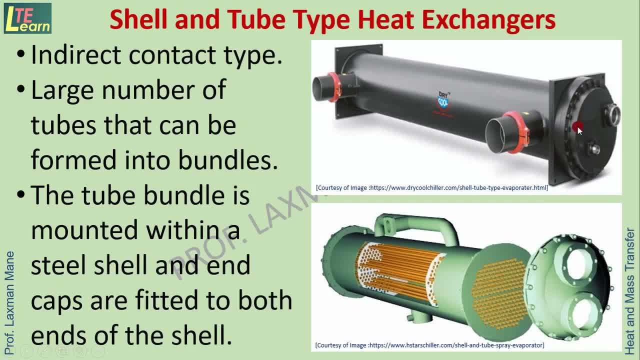 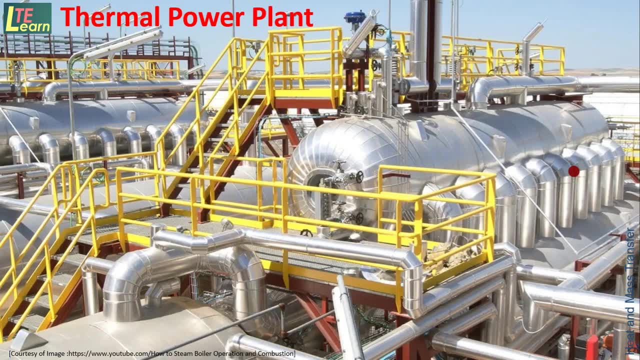 so this side of the shell is released and then it enters through to the other chest. These are the two caps which are fitted at the ends. This kind of heat exchangers are used in thermal power plant for condensation of steam from the boiler. 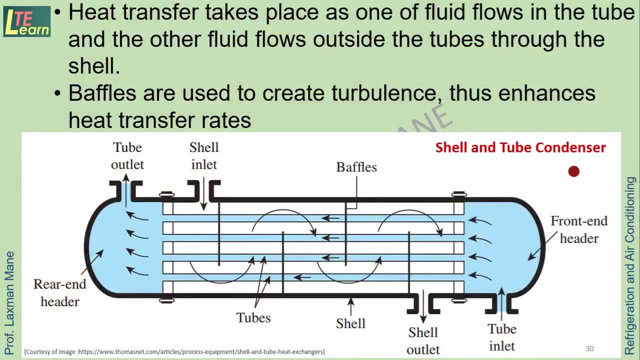 So here you can see this is a shell and tube condenser. In this heat transfer takes place as one of the fluid flows in the tube and other fluid flows outside the tubes through the shell. So here steam is passing shell side. It is condensed when it comes in contact with this water. 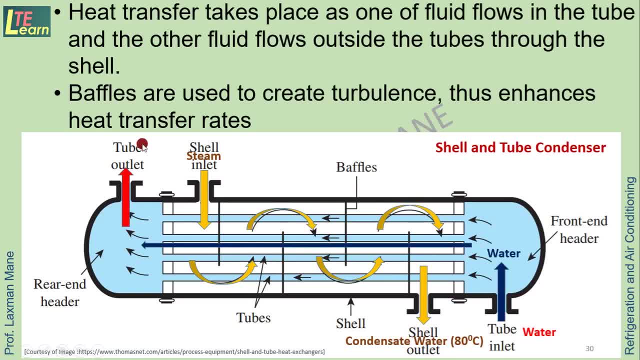 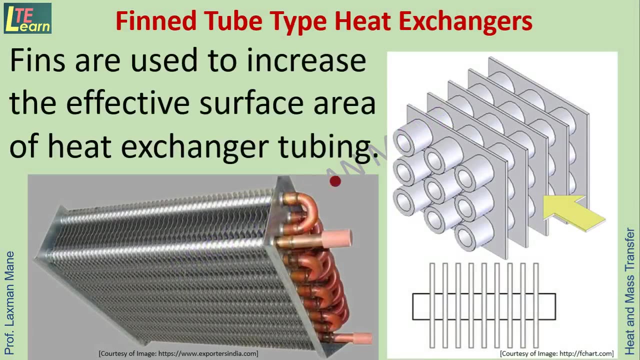 This water is coming out, So there is a heat exchange between steam and water. Okay, So here. baffles are used to create turbulence, thus enhances heat transfer rates. In case of finned tube type heat exchangers, fins are used to increase the effective surface. 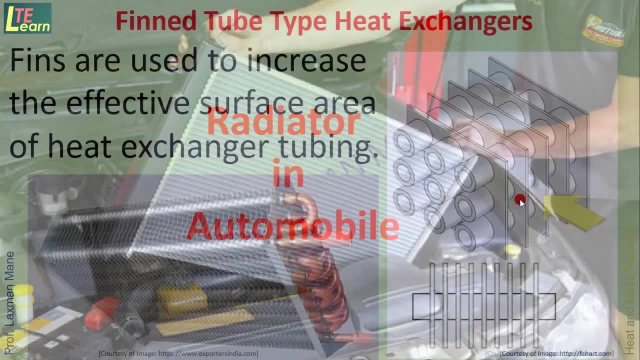 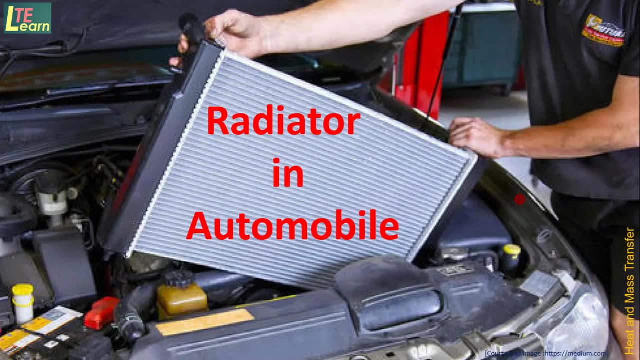 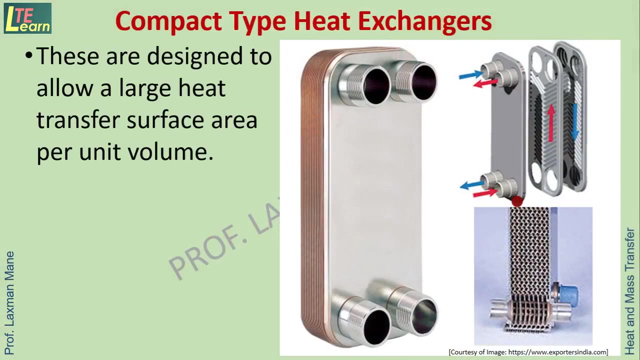 area of heat exchanger tubing. These are used as a radiator in automobile for cooling of oil of engine. Okay, Compact type heat exchangers, These are designed to allow a large heat transfer area per unit volume. So the ratio of heat transfer surface area of heat exchanger to its volume is called. 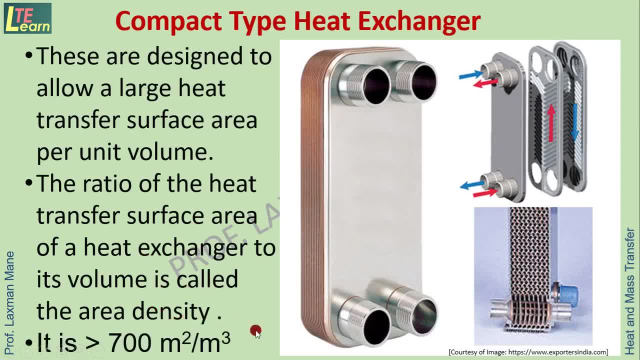 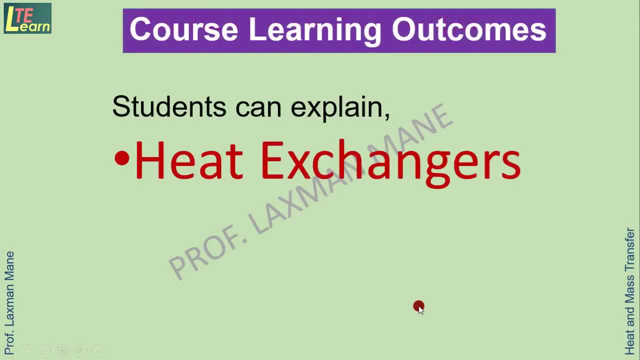 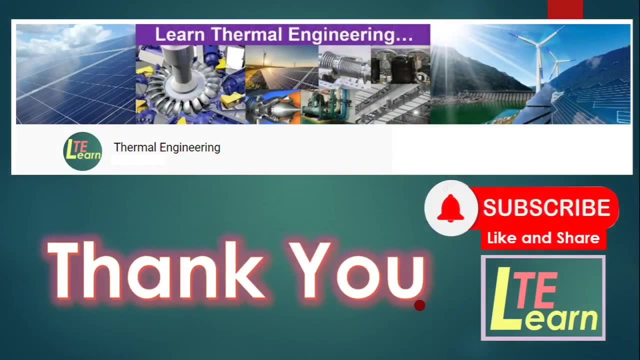 as area density, which is more than 700 m2 per m3.. So at the end of this session you can explain heat exchangers and its classification. Okay, So subscribe the channel for such kind of video sessions. Thank you.